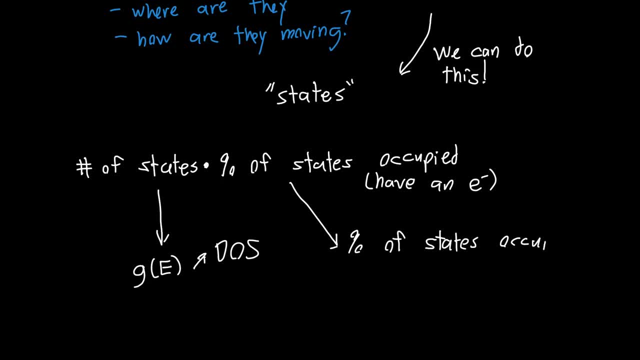 occupied and we would like to know the percentage of those states at a given energy, because we've got the density of states in terms of energy. so if we could multiply the density of states by the percentage of states that are occupied at a given energy, that gives us the 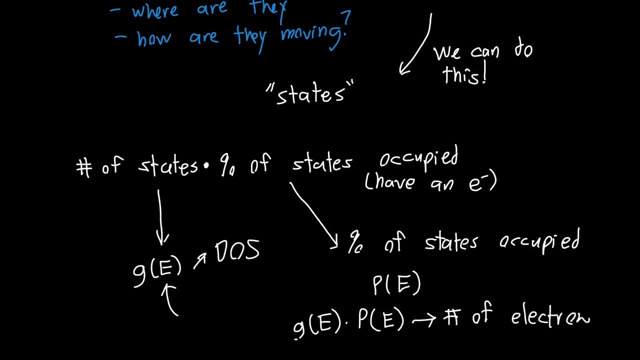 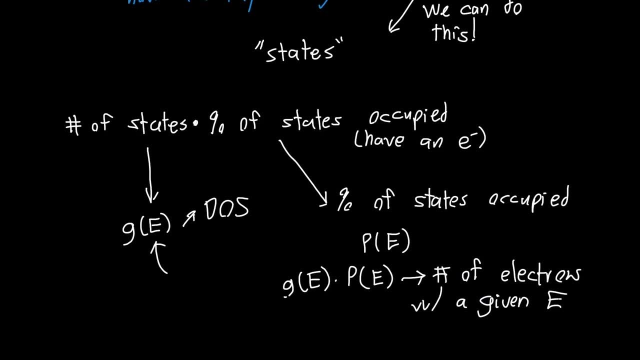 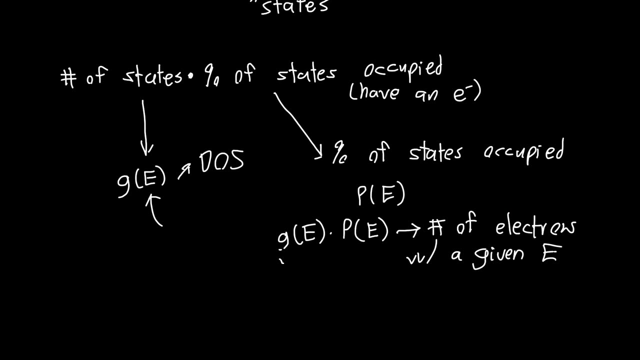 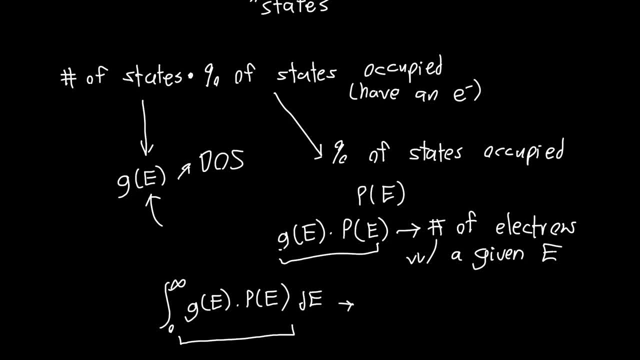 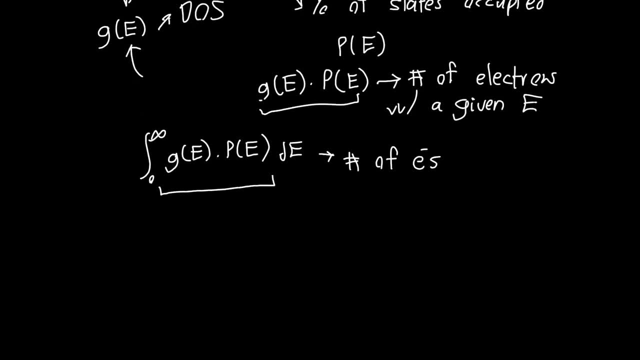 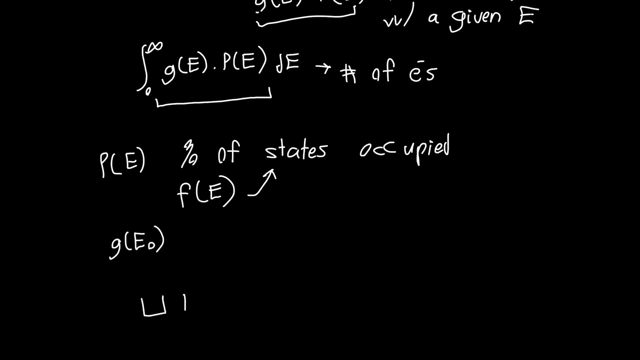 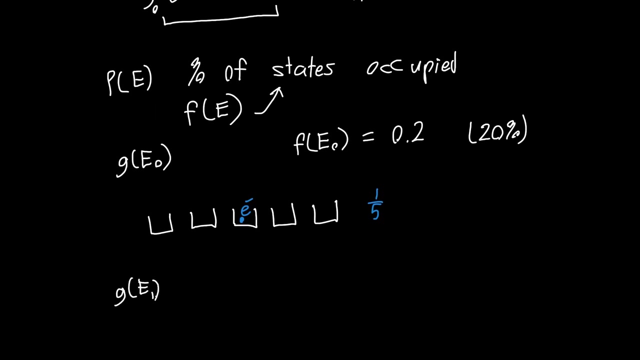 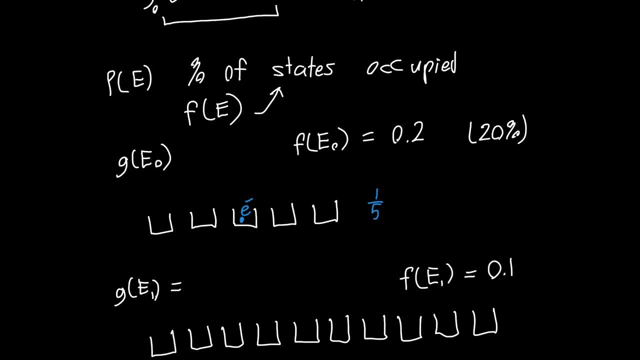 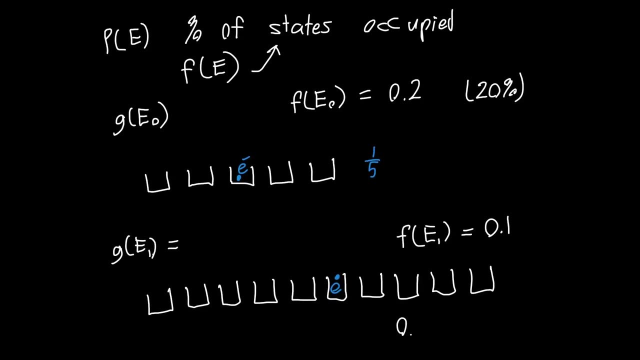 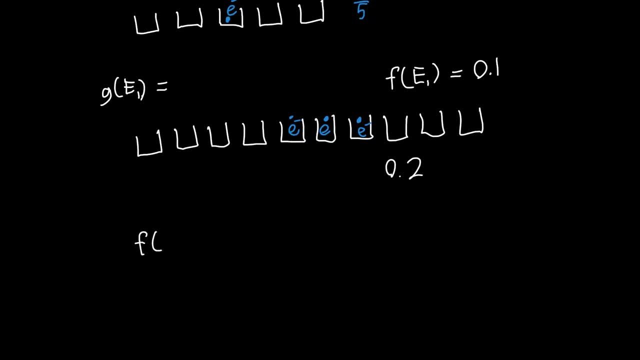 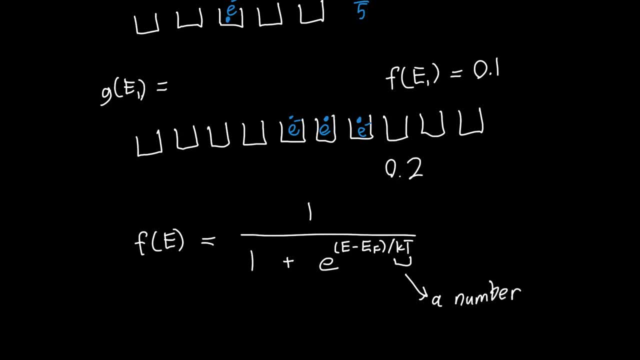 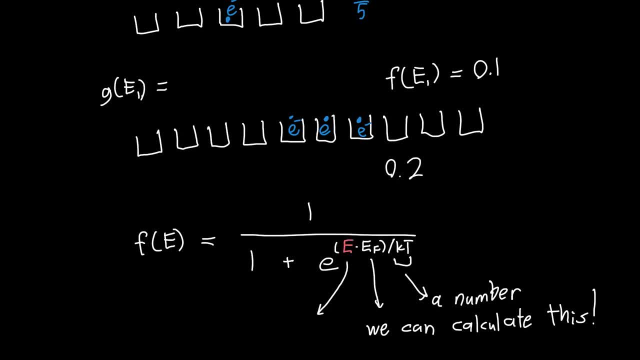 in red. so that's absolutely clear. this is the one variable in this entire function. this is the energy, and so this is the function. what does it look like? well, if you want to know what it looks like, it's helpful to draw it at some temperature. 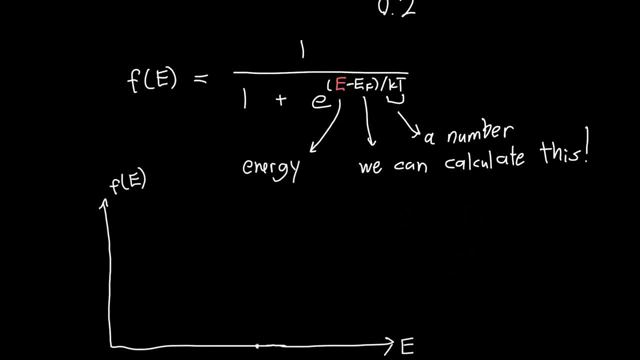 T. so let's just assume for now that T is room temperature, so about 300 Kelvin. then, since I've memorized this, I know that KT is about 26 milli electron volts. and so what does this function look like? at various or as we, as we? 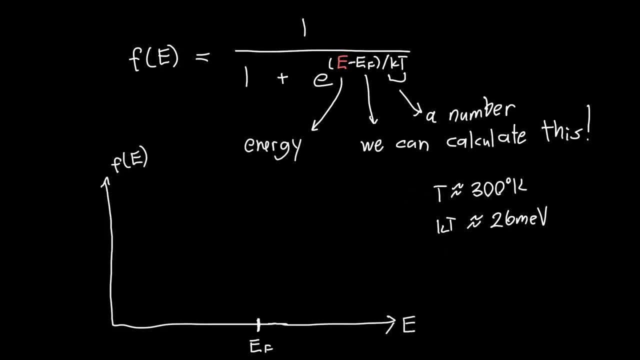 change E. well, let's call this position EF, because that's I mean that that's probably going to be special, right? so what does it look like when E is much, much less than EF, so, or when, say, E is equal to zero, for example? well then this: 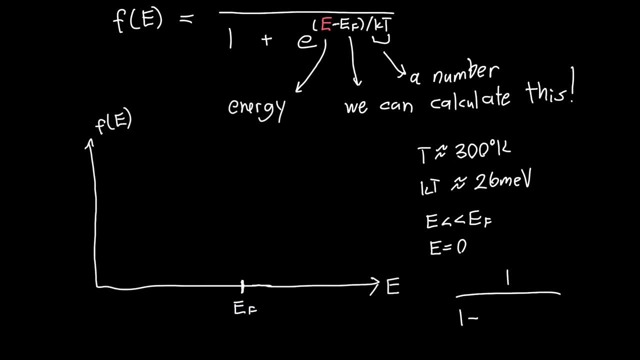 equation just looks like 1 over 1 plus E to the minus, EF over KT, and since I've done some semiconductor physics, I know that this EF is usually like 0.5 electron volts and 0.5 divided by 0.026 in this. 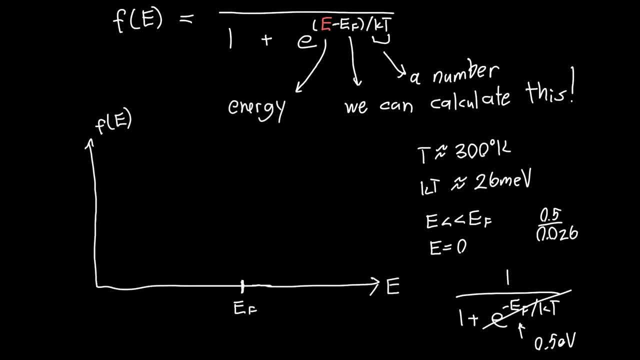 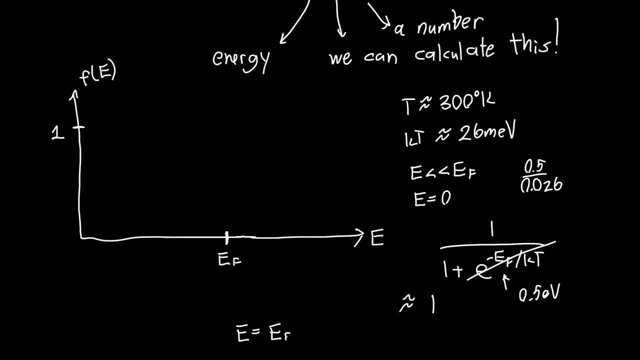 exponential term, this is gonna be very close to zero. so our Fermi function is approximately 1 and energy is much smaller than the Fermi energy. what about when the energy is equal to the Fermi energy? so E is equal to EF. well then this function just becomes 1 over 1, plus E to. 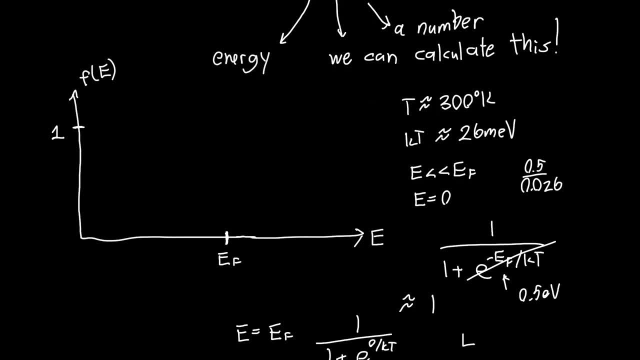 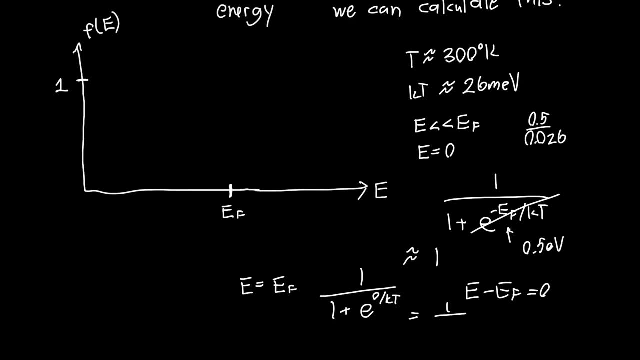 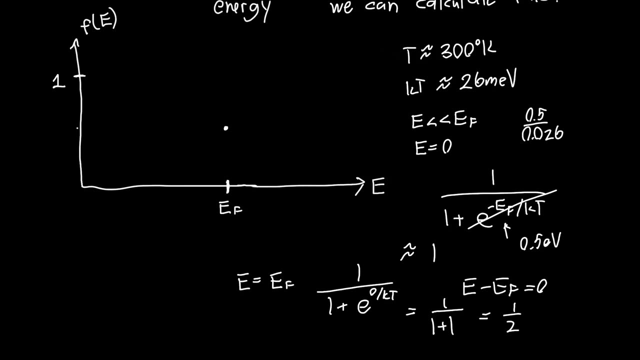 the zero over KT, because E is equal to EF. so E minus EF is just equal to zero. or 1 over 1 plus 1, which is just equal to 1 half. so when E is equal to EF, our Fermi function drops to 1 half. and now what a. 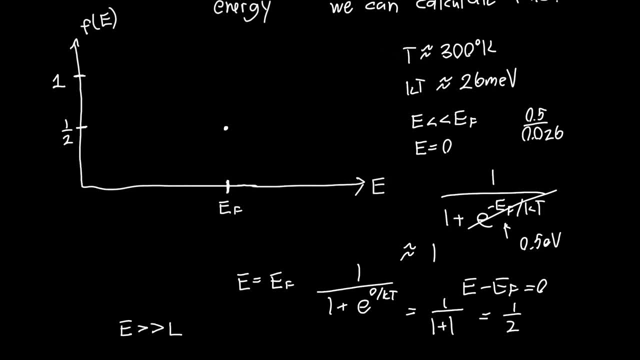 when E is much larger than EF. Well, we've got 1 over 1 plus E, to the some large number, let's say I don't know, like two electron volts, for example, divided by KT, which is 0.026 electron volts. This is a very large number because when we take 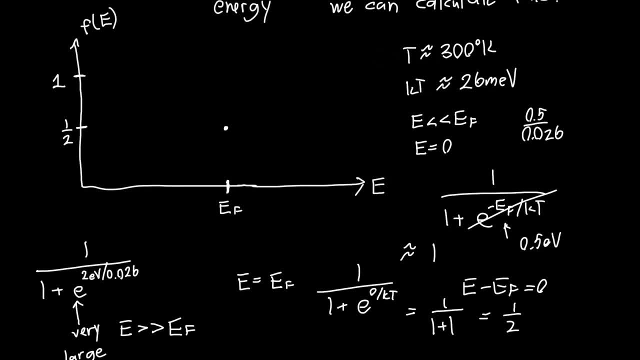 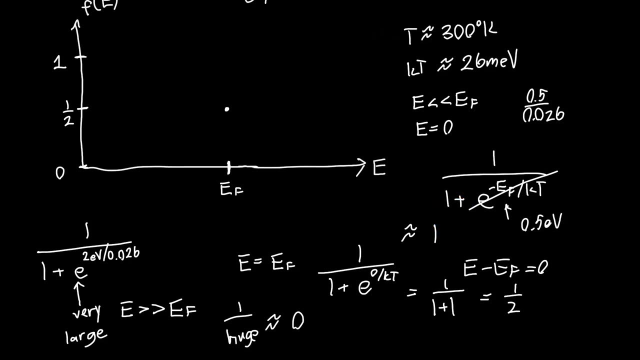 the exponential of some like number, like 10, 20, it's huge. So 1 over a huge number is just approximately 0.. So the Fermi function, when E is much greater than EF, is going to fall to 0.. And so we've got three points so we can kind of 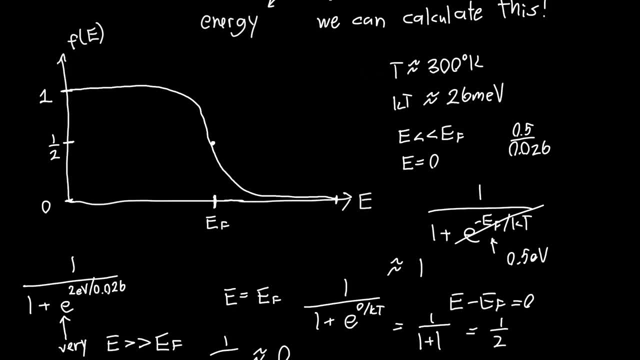 fudge it. We can say, okay, well, it's going to look something like this: So this is what the Fermi function is going to look like. So we've got three points. so we function looks like as a function of energy. Now let me just erase some of this. What about? 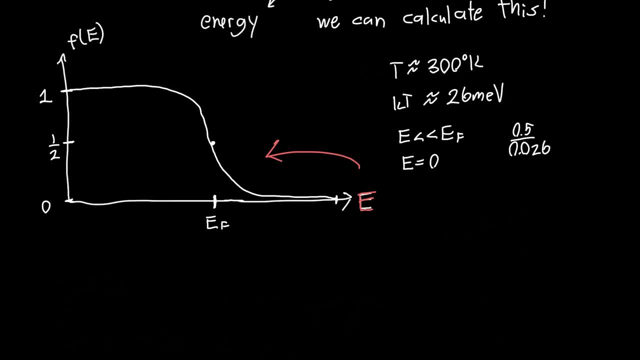 when we change the temperature. What happens to this function? What does it look like then? So we said that this was about, this was for. T is about I don't know, 300 Kelvin, 300 Kelvin. What happens when we reduce the temperature? Well, let's reduce it to something. 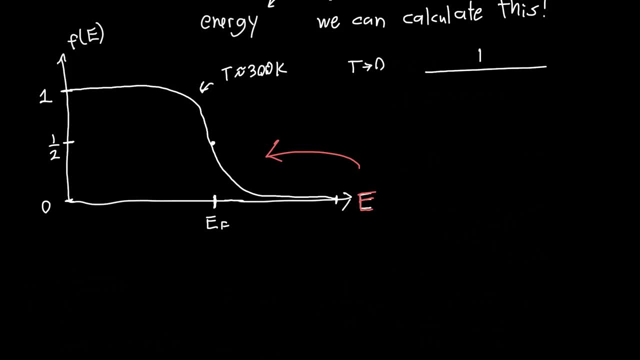 absurdly small. Let's say what if the temperature is equal to zero? Then the Fermi function is just one over one, plus e to the e minus ef over zero. And you might say: well, hold on a minute, Jordan, you can't do that. You've got a zero, one over zero in an exponential. That's nonsense. 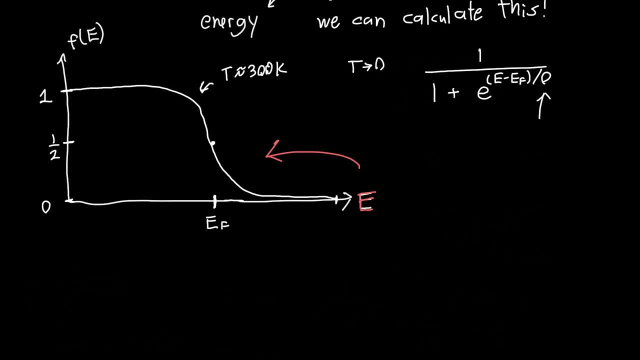 But to that I would answer: yes, I can do that, Because this is a ratio. So if you wanted you could take a limit. But essentially, um, when e now is less than the Fermi energy, this is one over one plus e to the. 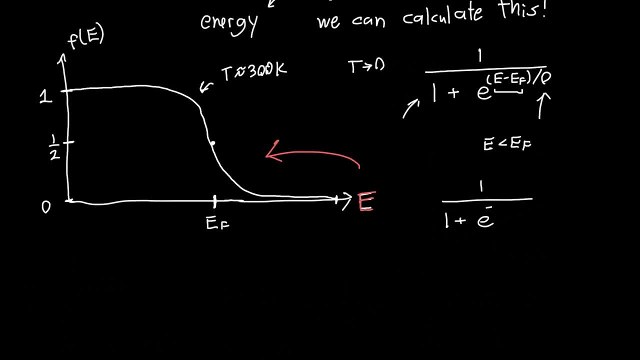 some constant number which is a negative, So it's some negative number divided by zero, which is just negative infinity. uh, approximately. So this just becomes one over one plus zero, because e to the minus infinity is zero, So this is just equal to one. Well, that's. 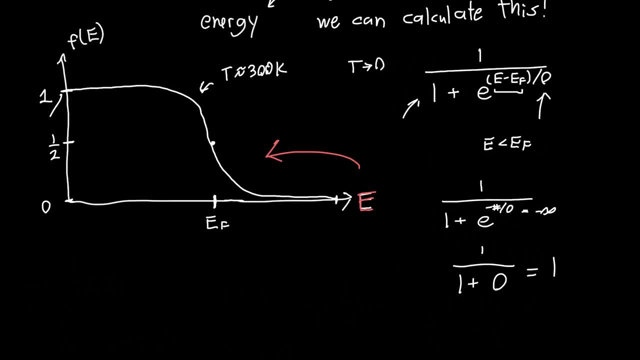 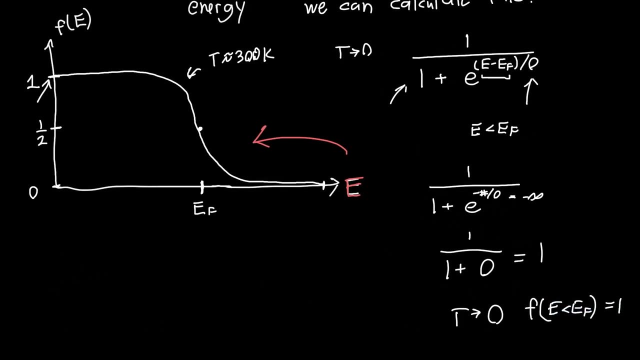 basically what we said before. So uh, approximately one, except as the temperature approaches zero. uh, f of f, when uh, e is less than ef, is exactly one. And that's kind of cool. Uh, what about when e is greater than ef? Well then, we've got the same situation. We've got one. 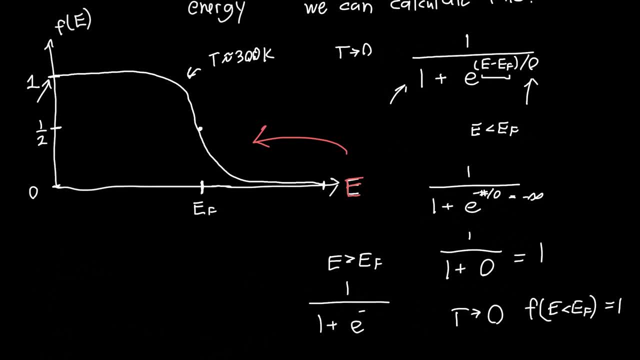 over one, plus e to the, now it's a positive number. So some positive number: e to the minus infinity is one over one, plus e to the minus infinity, which is zero. So instead of positive, negative infinity it's positive infinity And one over e to the infinity. 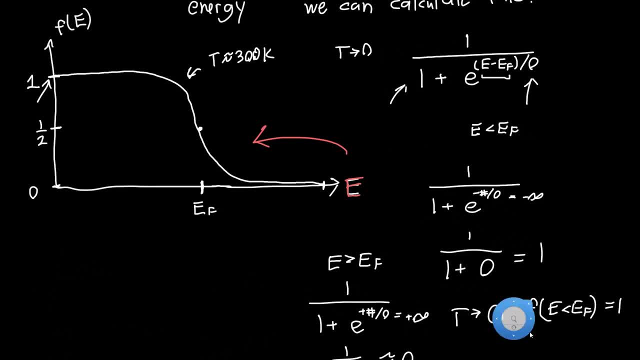 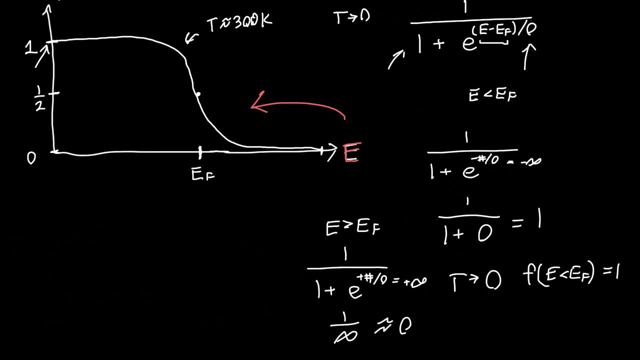 is just one over infinity which is zero, And I hope there's no mathematicians in the audience who I'm giving a heart attack right now- So the Fermi function immediately drops. So if t is equal to zero degrees Kelvin, it's one for e less than ef and zero for e greater. 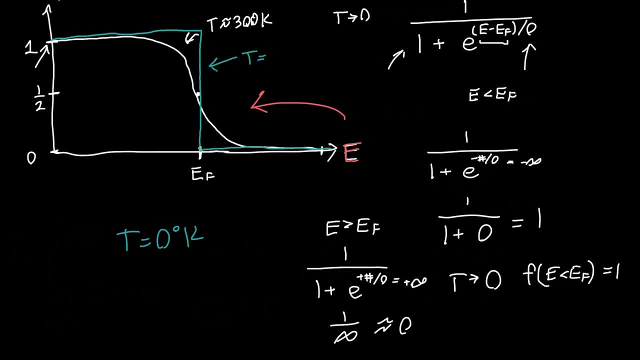 than ef. And so this is the temperature equal to zero degrees Kelvin. And so we can kind of get an intuitive sense for what's happening. As we raise the temperature, the Fermi function is kind of getting smoothed out. So if we were to say t is equal to a thousand Kelvin, the Fermi function